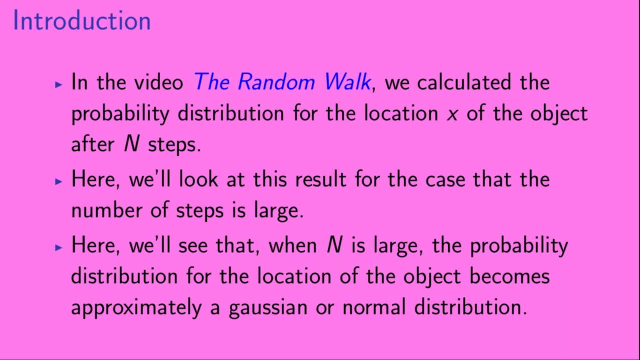 for the location x of the object after n steps. Here we'll look at this result for the case that the number of steps is large. Here we'll see that when n is large, the probability distribution for the location of the object becomes approximately a Gaussian or normal. 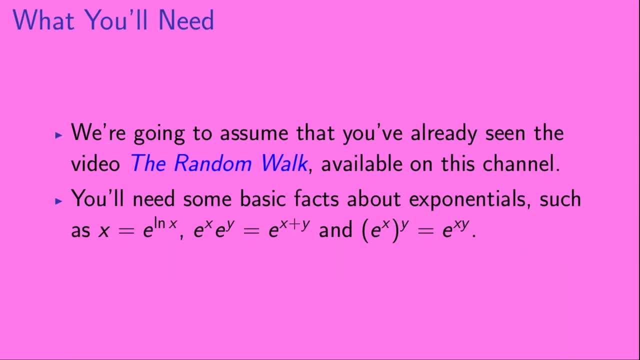 distribution. There are a few things you're going to need for this video, so we're going to assume that you've already seen the video, the random walk- available on this channel. You'll also need some basic facts about exponentials, such as the fact that x equals e raised to the power of the natural log of x and e to the x. 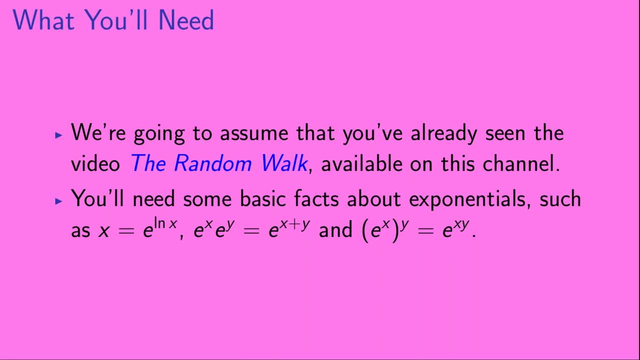 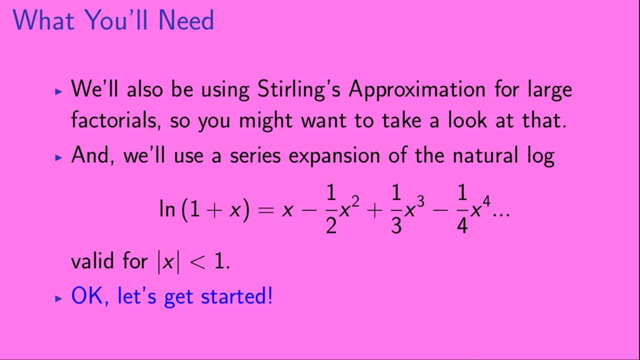 times e to the y equals e to the power of x plus y and that e to the x power raised to the y power equals e to the power of xy. We'll also be using Stirling's approximation for large factorials, so you might want to take a. 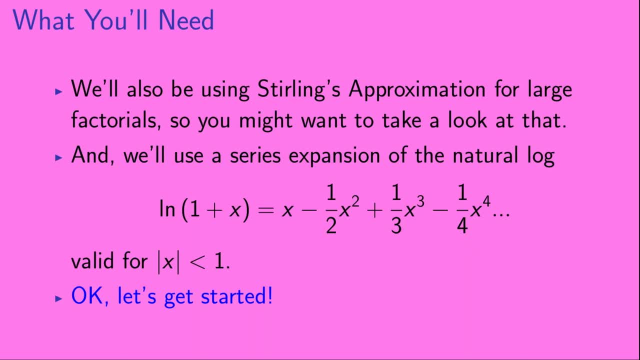 look at that before continuing. And also we'll use a series expansion of the natural log. So the natural log of one plus x is equal to x minus one half x squared, plus one third x cubed, etc. as long as the absolute value of x is less than one. Okay, so with that let's get started. Okay, so our 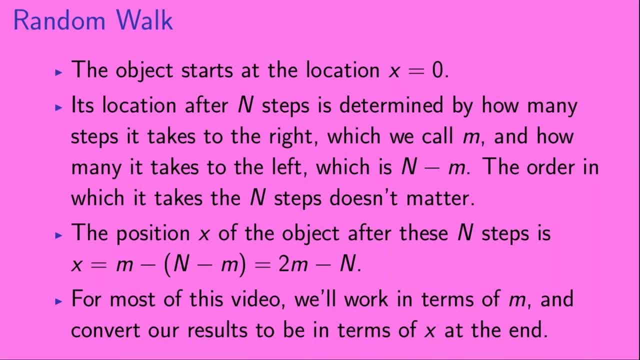 object is defined to be a Castel mode. that's very easy to founders. The argument is: we'll use a staged search method here. We're going to look at a random walk and find something worth solving, And the reason we use this is because the number of steps in the row that we do is 0.. 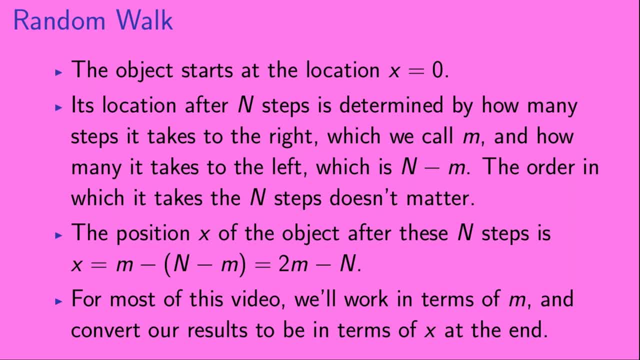 which is m minus the number of steps to the left, which is n minus m. So x equals 2m minus n. For most of this video, we'll work in terms of m and convert our results to be in terms of x at the end. 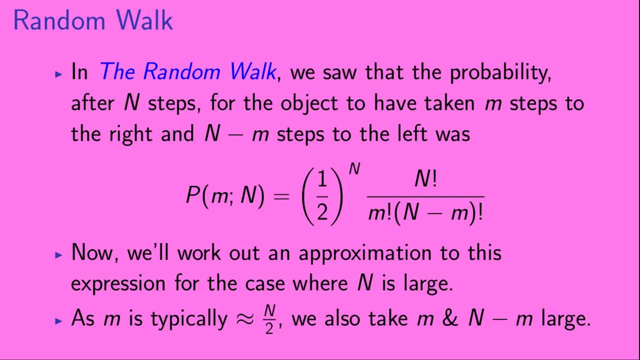 In the video The Random Walk, we saw that the probability, after n steps, for the object to have taken m steps to the right and n minus m steps to the left was given by what we called p of m. given n, which equals 1 half to the n power times. n factorial over m factorial. n minus m factorial. 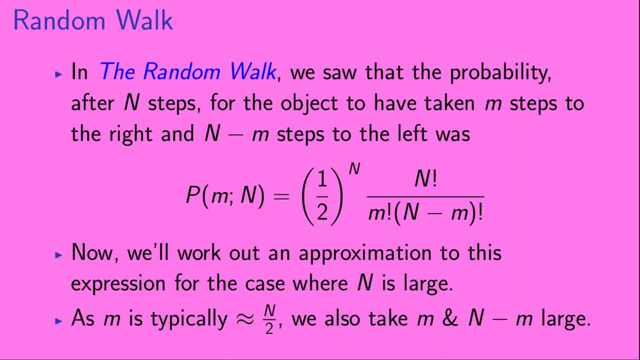 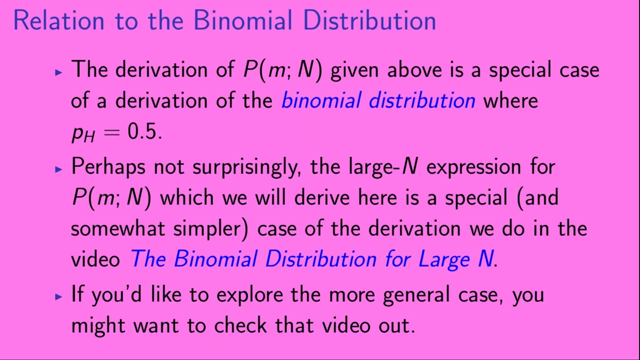 Now we'll work out an approximation to this expression for the case where n is less, As m is typically about n over 2, we will also take m and n minus m as large The derivation of p of m given n, as shown above. 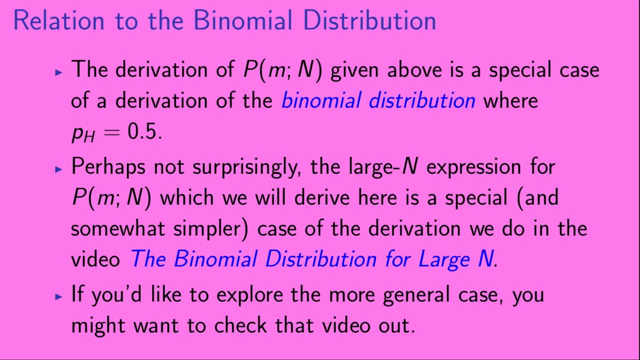 is a special case of a derivation of the binomial distribution where pH equals 0.5.. Perhaps not surprisingly, the large n expression for p of m, given n, which we will derive here, is a special and somewhat simpler case of the derivation we do in the video. 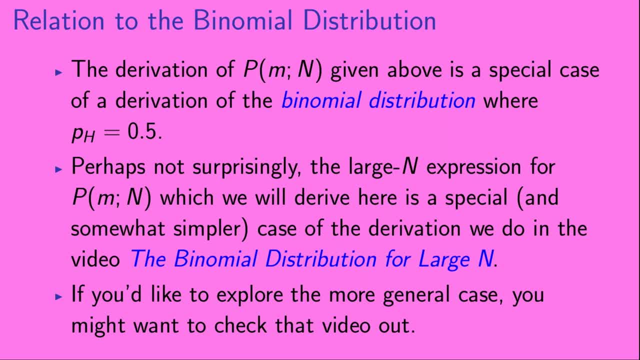 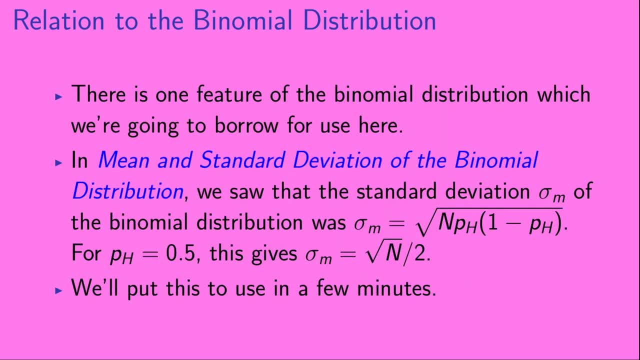 The Binomial Distribution for Large N. If you'd like to explore the more general case, you might want to check that video out. There is one feature of the binomial distribution which we're going to borrow for use here In the video: Mean and Standard Deviation of the Binomial 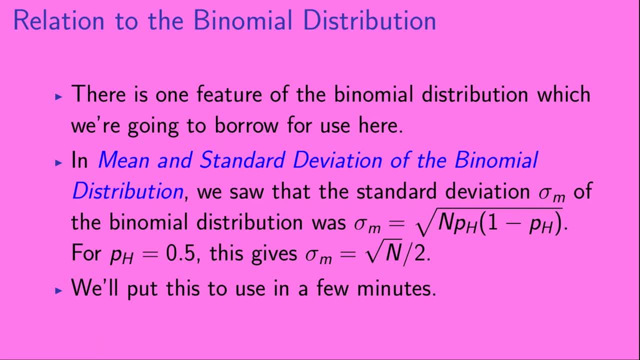 we saw that the standard deviation sigma m of the binomial distribution was given by. sigma m equals the square root of n pH, 1 minus pH. For the case pH equals 0.5, this gives sigma m equals the square root of n over 2.. 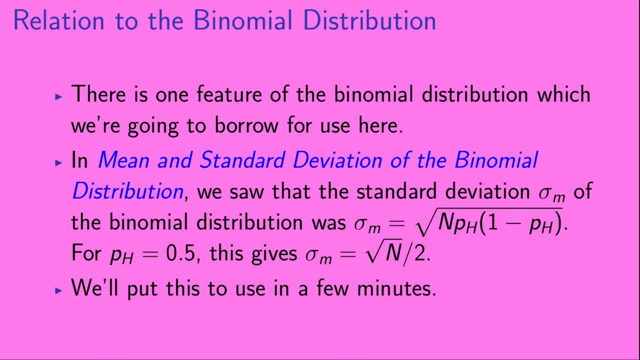 We'll put this to use in a few minutes, So we'll use this equation to find the square root of n. We'll use this equation to find the square root of n. We'll use this equation to find the square root of n. 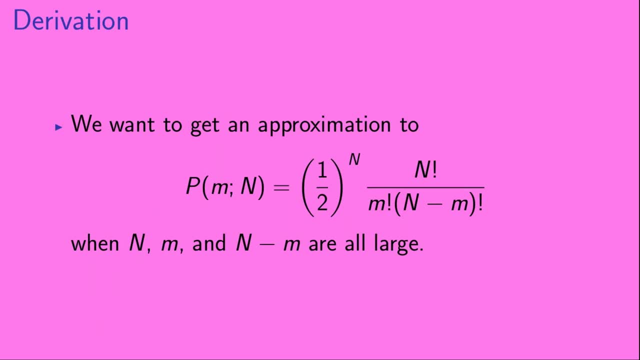 So we want to get an approximation to our expression for p of m given n, which was 1 half to the n times n factorial over m factorial, n minus m factorial for the case when n? m and n minus m are all large. 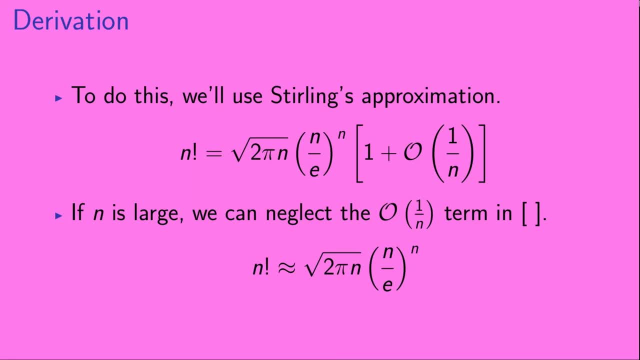 To do this, we're going to make use of Sterling's approximation for large factorials. To do this, we're going to make use of Sterling's approximation for large factorials. So Sterling's approximation tells us that n factorial is equal to the square root of 2 pi n times n over e raised to the n power. 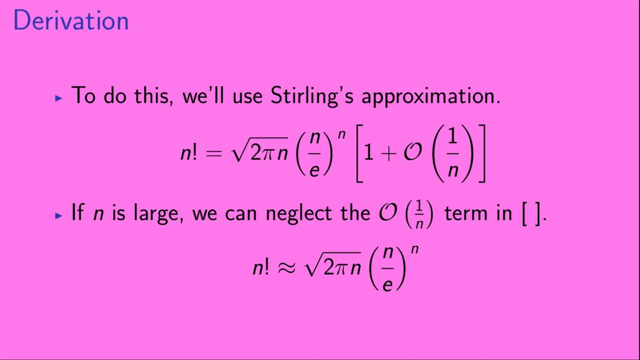 times 1 plus terms of order 1 over n. If n is large, we can neglect the terms that are of order 1 over n inside the brackets, And so we have: the n. factorial is equal to the square root of 2 pi n times n over e, raised to the n power times 1 plus terms of order 1 over n. And so we have the n factorial is equal to the square root of 2 pi n times n over e, raised to the n power times 1, plus terms of order 1 over n. And so we have the n factorial is equal to the square root of 2 pi n times n over e, raised to the n power times 1, plus terms of order 1 over n. 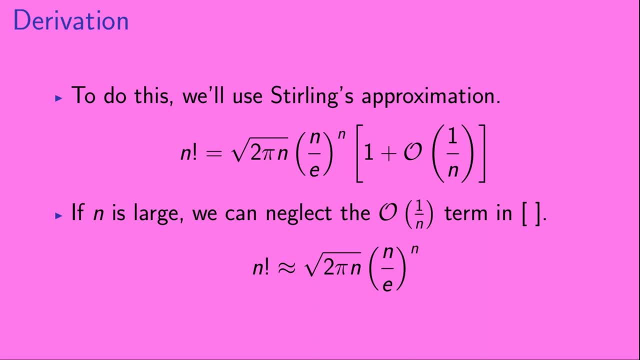 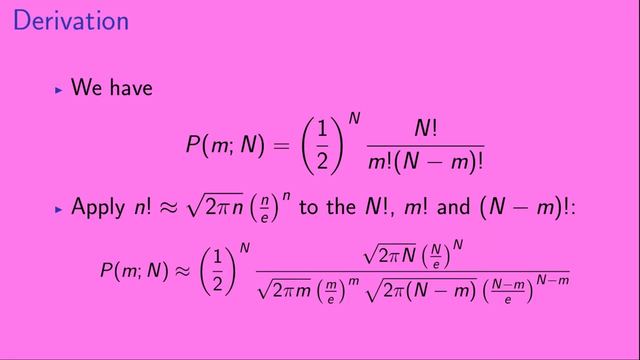 is approximately equal to the square root of 2 pi n times n over e raised to the n power. Okay, so our expression for p of m given n contains three factorials: an n factorial, an m factorial and an n minus m factorial. So now we're going to. 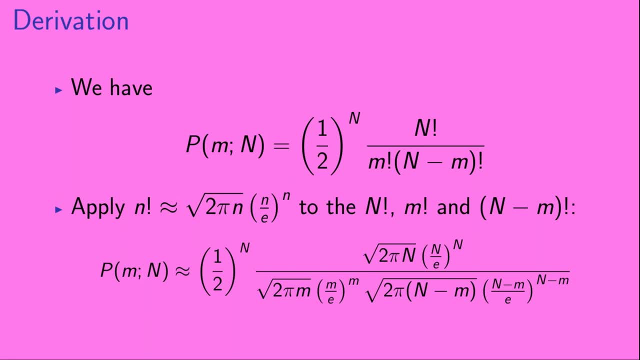 apply Sterling's approximation to the n factorial, the m factorial and the n minus m factorial in this expression. Okay, so on top we have an n factorial. This is going to become the square root of 2 pi n times n over e raised to the n. 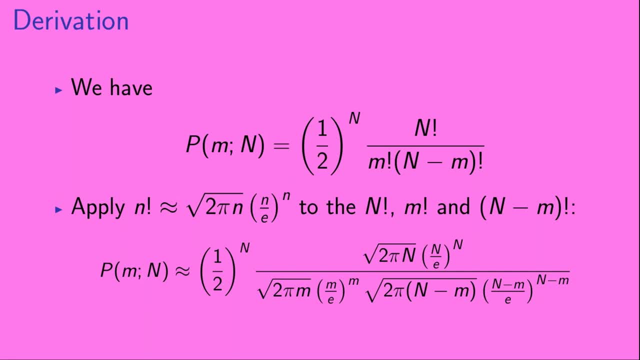 power. Next, in the denominator we have an m factorial. This becomes the square root of 2 pi m m over e to the m power. And also in the denominator we have an n minus m factorial. This becomes the square root of 2 pi n minus m times n. 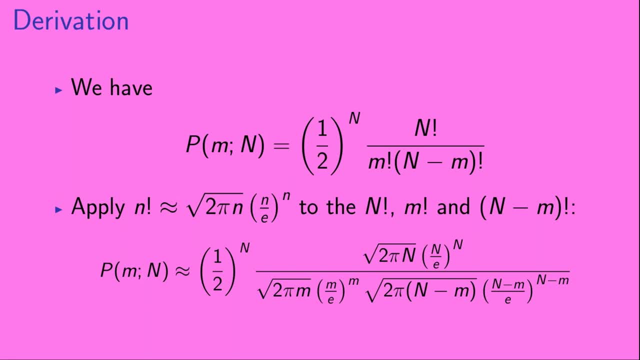 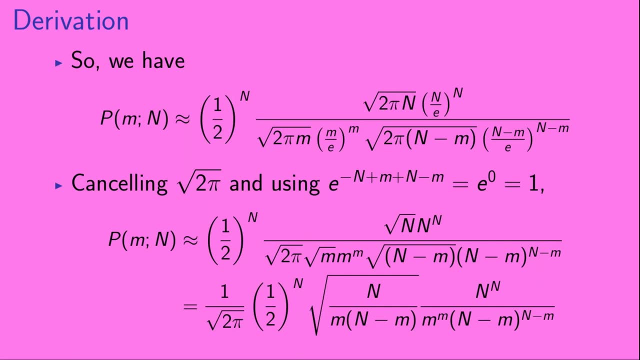 minus m over e raised to the power of n minus m. Okay, so now we have our expression for p of m given n, just copied from the previous slide. Now we're going to do two quick things. First of all, we're going 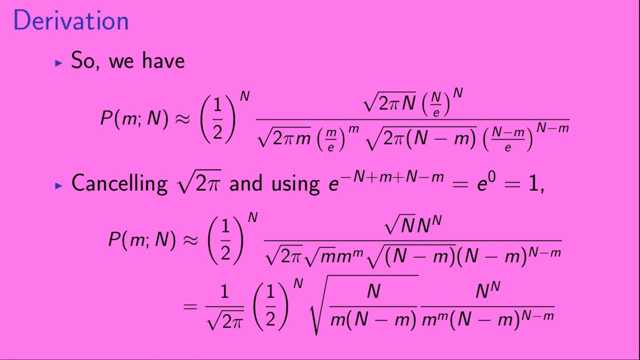 to cancel a factor of the square root of 2 pi from the numerator and the denominator in this expression, leaving just one factor of the square root of 2 pi in the denominator. Next we can look at the factors of e in this expression. 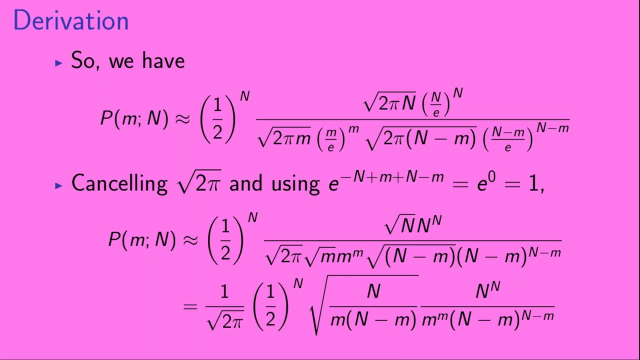 So in the numerator we have an e to the minus n power and in the denominator we have an e to the minus m power and an e to the minus n minus m power. If we put all of those together we get e to the minus n plus m, plus n minus m. 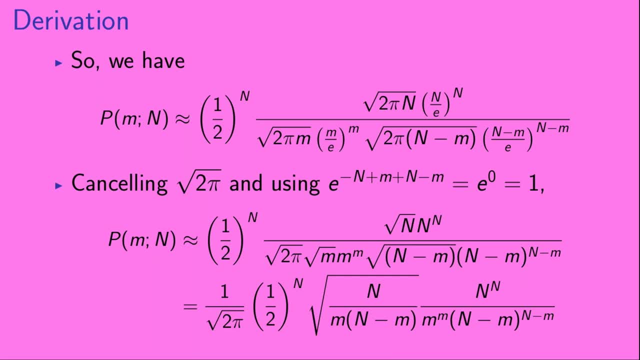 which is just e, to the zero, which just equals one. So we can cancel out all of those factors of e. So we get that p of m, given n, is approximately equal to one half to the n times the square root of n times n to the n. 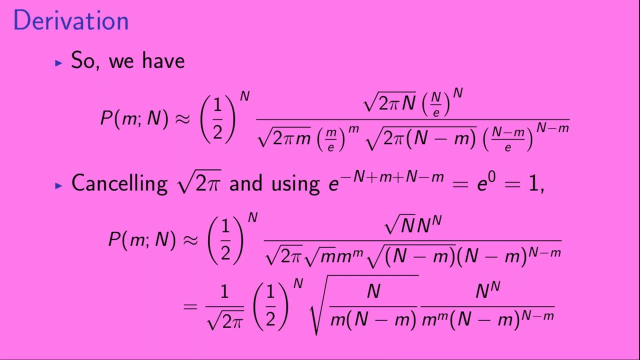 over the square root of two pi. the square root of m m to the m times. the square root of n minus m times n minus m to the n minus m power. Now we can make this look slightly prettier by collecting all of those square roots together. 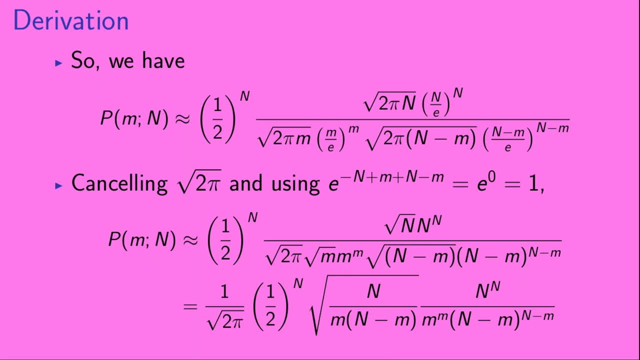 and so we get that p of m, given n, is approximately equal to one over the square root of two pi. one half to the n times the square root of n over m, n minus m times n to the n over m to the m. 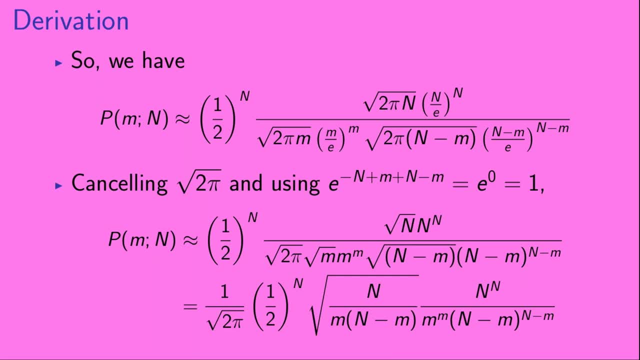 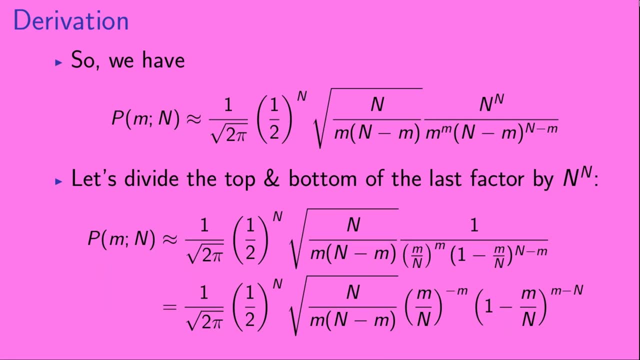 n minus m to the power of n minus m. Okay, so now we have our expression for p of m given n. Let's take a look at the last factor in this expression: the n to the n over m to the m. 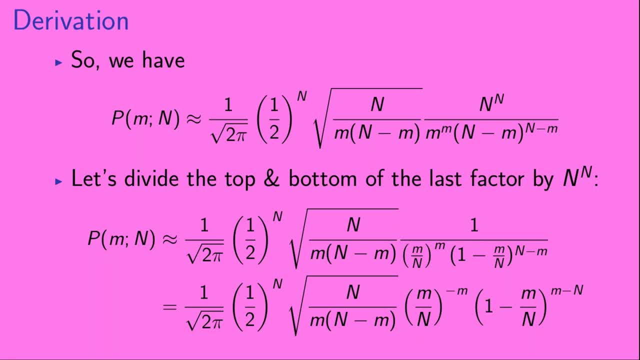 n minus m to the n minus m. Let's divide the top and bottom of this last factor by n to the n. So in the numerator we get n to the n. divided by n to the n, that just gives one. In the denominator we can get m over n to the m power. 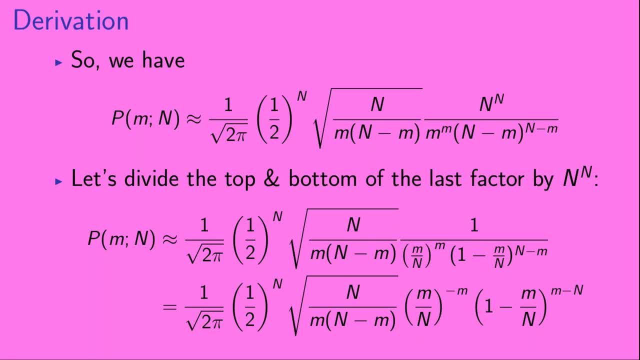 times one minus m over n, raised to the power of n minus m. And now we can make this a little bit prettier by writing one over m over n to the m power as m over n to the minus m, and writing one over 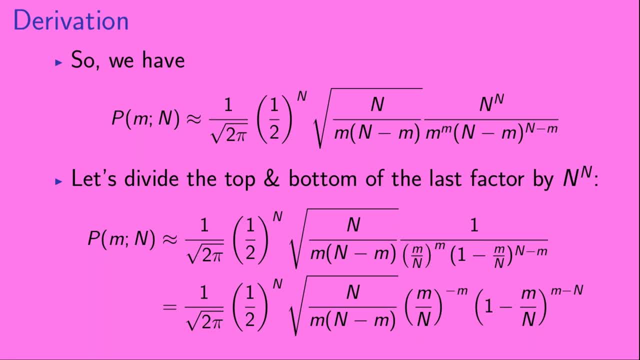 one minus m over n to the n minus m power, as one minus m over n to the n minus n power. So now we get that p of m, given n is approximately equal to- Let's do the math to- the power of 1 minus m over n. 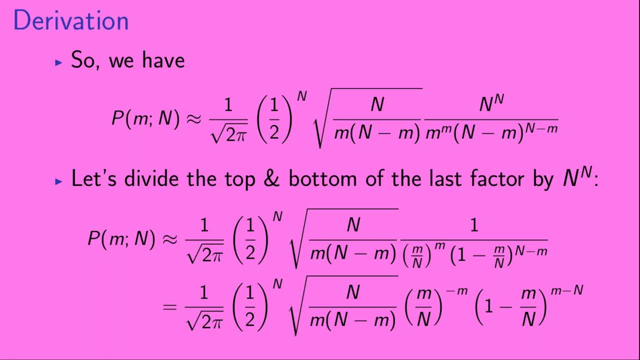 to the n minus m power equal to 1 over the square root of 2 pi 1. half to the n times the square root of n over m n minus m times m over n. to the minus m power times 1 minus m over n. 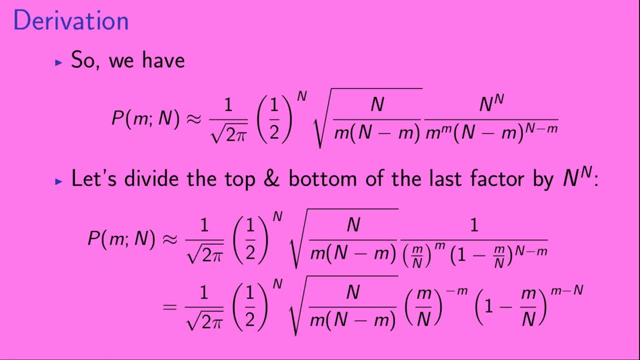 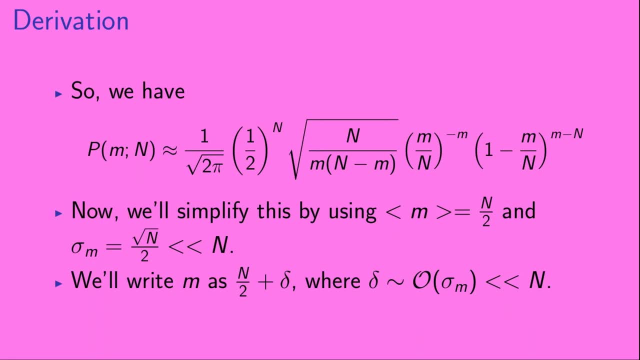 to the power of m minus n. Okay, so now we have our expression from the previous slide. Now we can simplify this by using the fact that the mean value of m is equal to n over 2, and the standard deviation of m sigma m is equal to the. 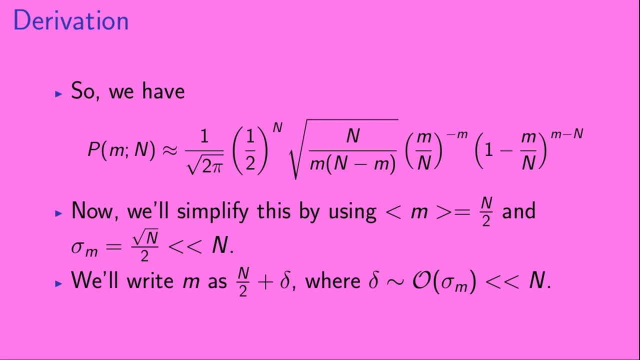 square root of n over 2, and that's much less than n. So the standard deviation of m tells us approximately, typically, how much m differs from its mean value of n over 2.. So we can write m as n over 2 plus delta, where delta is of the. 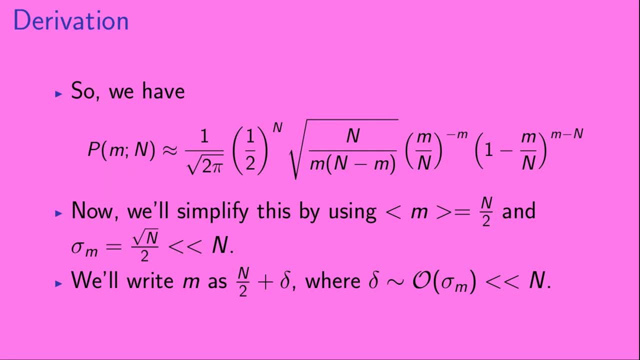 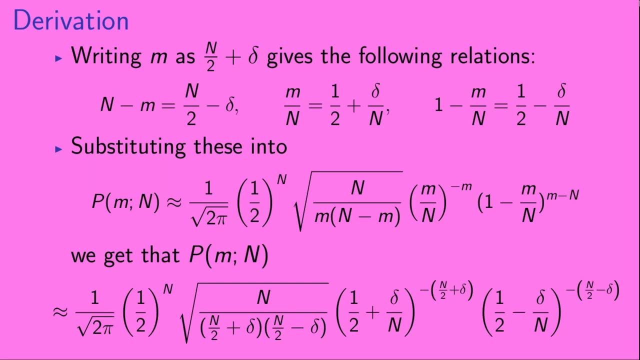 order of sigma m, which is much less than n. Okay, so writing m as n over 2 plus delta gives the following three relations. First, n minus m is equal to n over 2 minus delta. Second, m equals n to the Cynthia 1942.. Next we get to cancel m. So the Какes-Z он или. 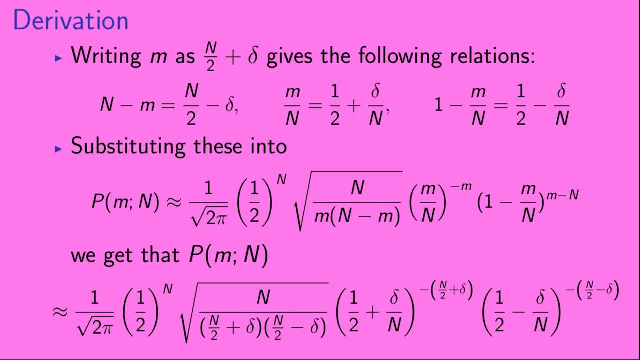 m over n is equal to 1 half plus delta over n. And third, 1 minus m over n is equal to 1 half minus delta over n. Now let's substitute these three relations into our expression for P of m, given n. 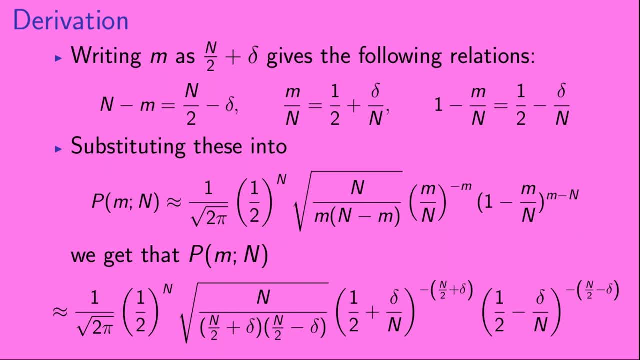 Let's look at each factor in P of m given n individually and see how this works out. So first, out front, we have 1 over the square root of 2 pi times 1, half to the n power. These factors are unaffected by our relations, so they just go through unchanged. 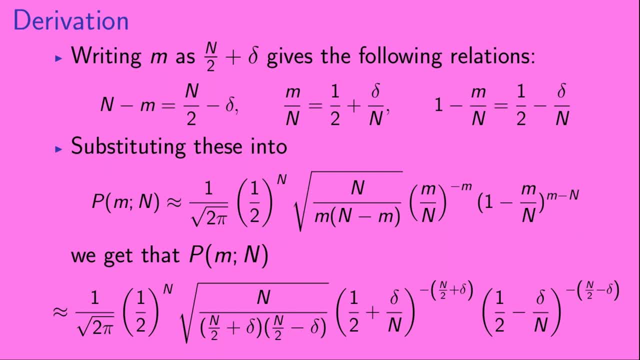 Next we have a square root, The square root of n over m, n minus m. This becomes the square root of n over n over 2 plus delta, n over 2 minus delta. So we've substituted in our relations for m and n minus m in the square root. 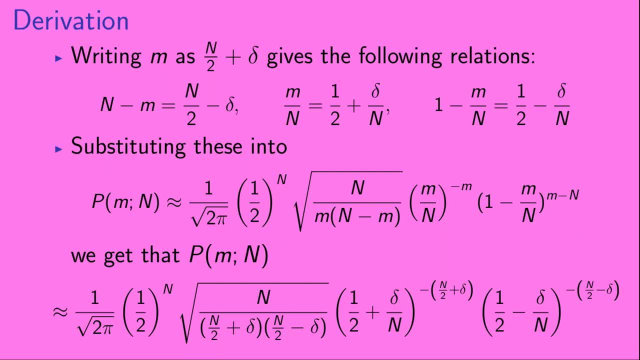 Next we have a factor of m over n raised to the minus m power. So we substitute in our relation for m over n, That's m over n equals 1 half plus delta over n, And in the exponent our expression for m. So minus m becomes minus n over 2 plus. 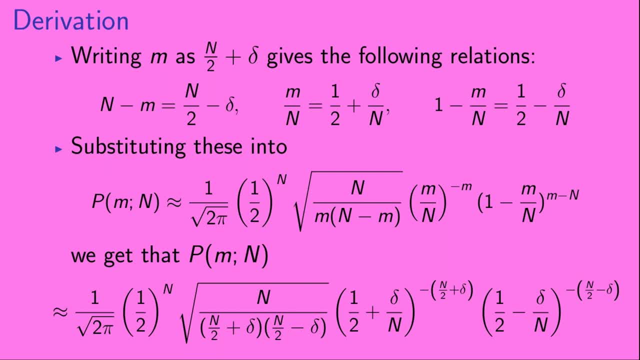 delta. Okay, now let's look at the last factor. in p of m, given n, We have 1 minus m over n, raised to the power of m minus n. 1 minus m over n equals 1 half minus delta over n. So we substitute that in and in. the exponent m minus n becomes: 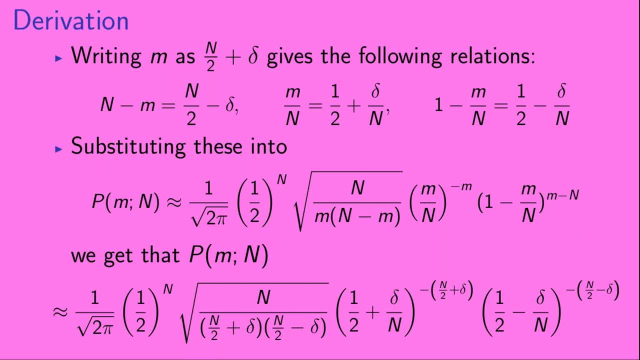 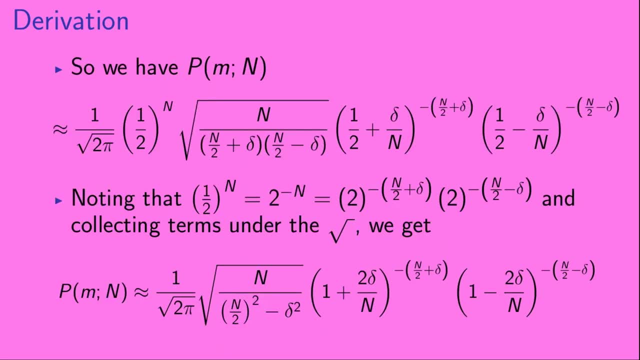 minus n, over 2, minus delta. Okay, now let's go on. Okay, so we have our new expression for p of m given n from the previous slide. Now we're going to do two simple things. First, we're going to look at that. 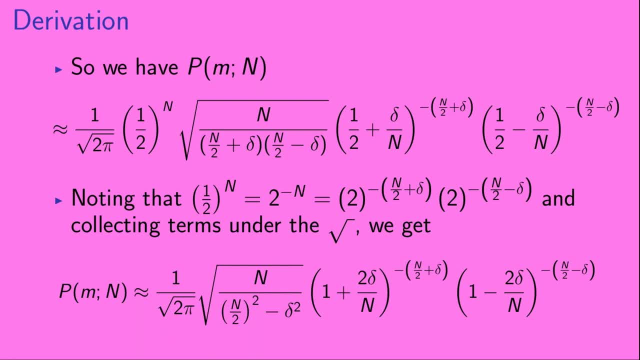 factor of 1 half to the n. that's out front. 1 half to the n is equal to 2 to the minus n, And 2 to the minus n is equal to 2 to the minus n over 2 plus delta times 2 to the minus n over 2 minus delta. So we can take these factors. 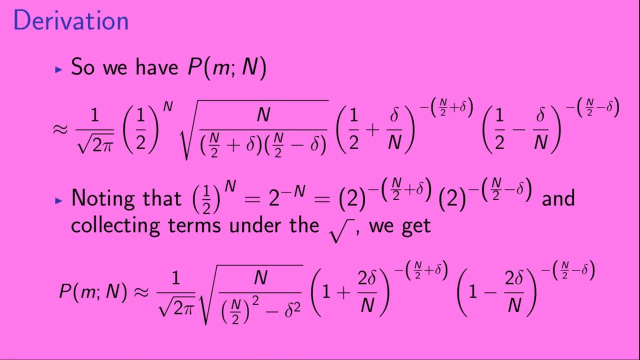 of 1 half and use them to simplify our last and next-to-last factors in our expression for p of m given n. Next, we can take the factors of n over 2 plus Delta and n over 2 minus Delta that are inside the square root. 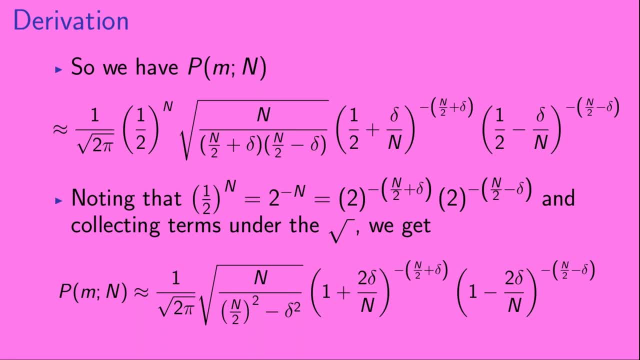 and we can multiply them out. So doing these two things, we get that p of m given n is approximately equal to 1 over the square root of 2 pi times the square root of n over n over 2 squared minus Delta squared times 1 plus 2 Delta over. 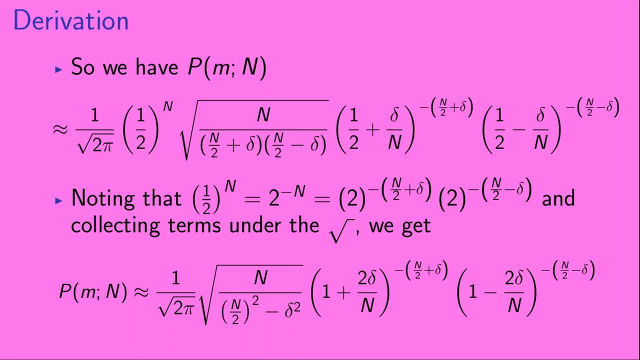 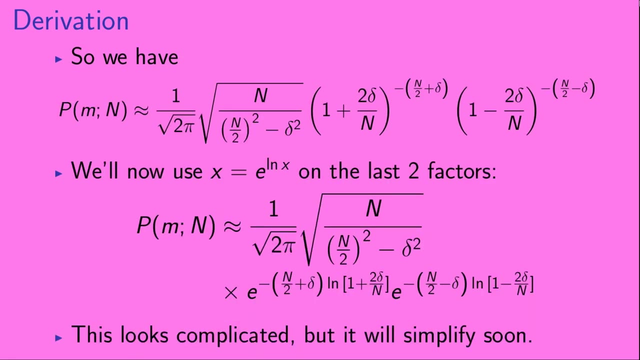 n raised to the power of minus n over 2 plus Delta times 1 minus 2 Delta over n raised to the power of minus n over 2 minus Delta. So we have our expression for p of m given n over 2 minus Delta, squared times 1 plus 2 Delta over n. 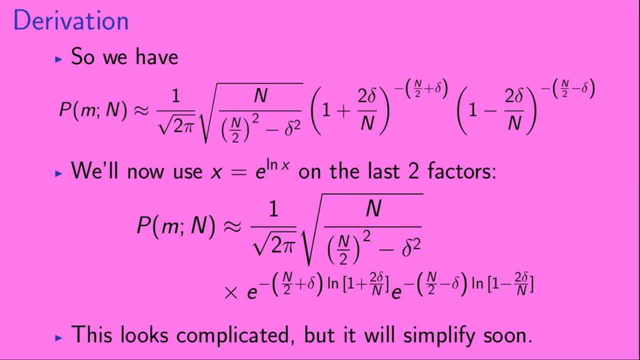 from the previous slide. Right now we're going to look at the last two factors in this expression. So we have 1 plus 2 Delta over n raised to some power and 1 minus 2 Delta over n raised to another power. We're going to use the relation x. 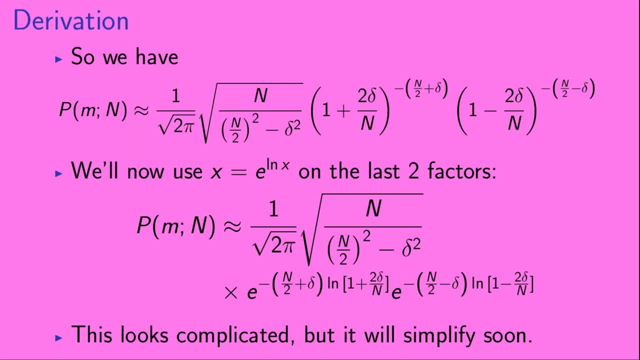 equals e raised to the power of the natural log of x on these last two factors. So we're going to write 1 plus 2 Delta over n as e raised to the power of the natural log of 1 plus 2 Delta over n, and we're going to write 1 minus 2 Delta over. 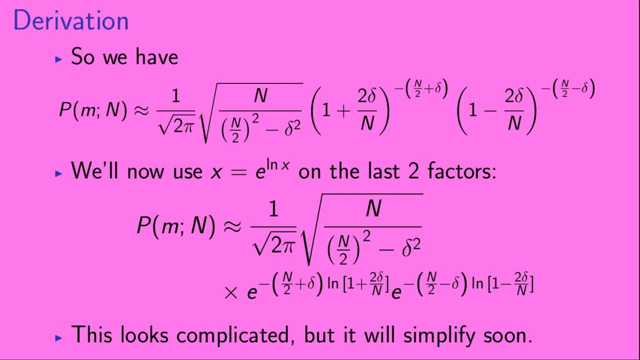 n as e raised to the power of the natural log of 1 minus 2 Delta over n. Now those last two factors are each raised to a power, so we have to take that into account as well. So what we get is that p of m given n is approximately equal to 1 over the square root of 2 pi times. 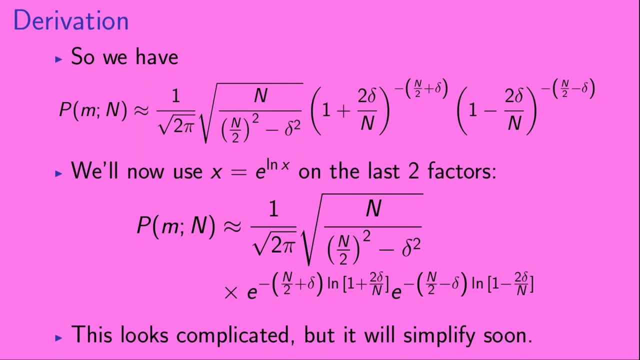 the square root of n over n over 2 squared minus Delta. squared times e to the minus n over 2 plus Delta. Natural log of 1 plus 2 delta over n times e to the minus n over 2 minus delta. natural log of 1 minus 2 delta. 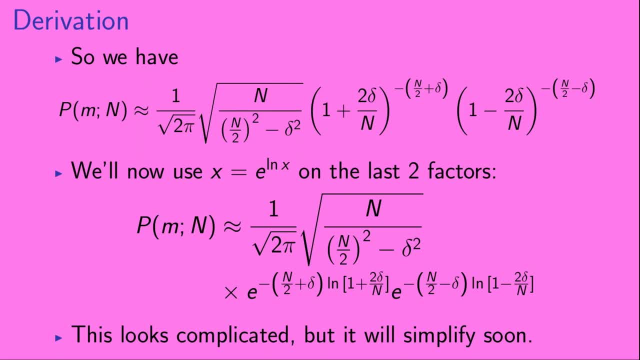 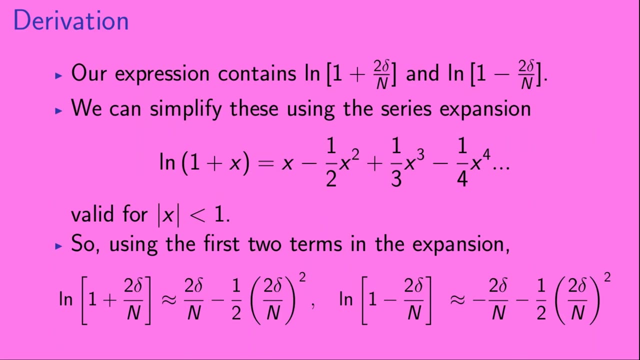 over n. Now this looks complicated and probably looks more complicated than what we had before, but it will simplify down a lot quite soon. So our expression contains factors of the natural log of 1 plus 2 delta over n and the natural log of 1 minus 2 delta over n. We can simplify these. 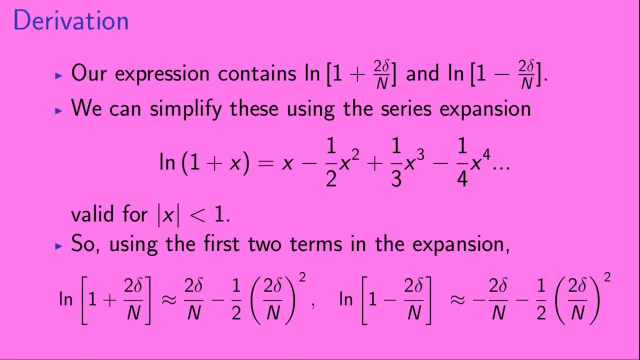 using the series expansion of the natural log of 1 plus x. So the natural log of 1 plus x, x equals x minus 1, half x squared plus 1 third x cubed, etc. as long as the absolute value of x is less than 1.. 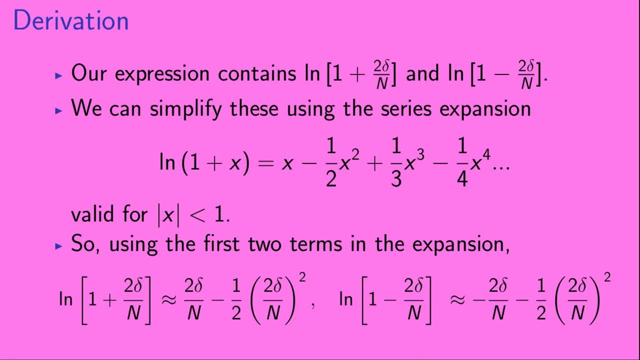 So using the first two terms in this series expansion, we can get that the natural log of 1 plus 2 delta over n is approximately equal to 2 delta over n minus 1, half the square of 2 delta over n. And the natural log of 1 minus 2 delta over n is approximately equal to minus 2 delta. 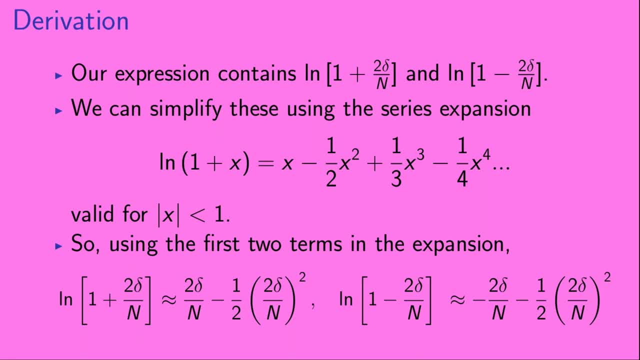 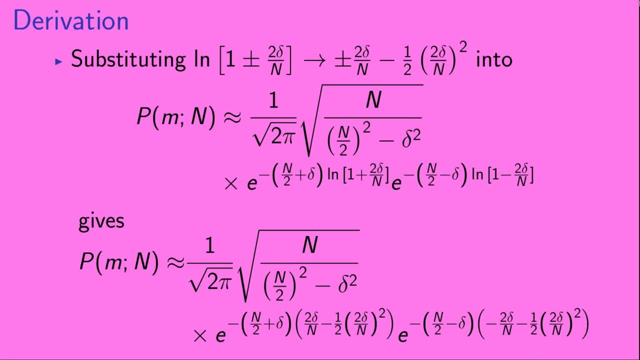 over n minus 1, half the square of 1.. So now we can take our approximations for the natural log of 1 plus or minus 2 delta over n and substitute them into our expression for P of m given n. So our expression for P of m given n contains two exponentials. 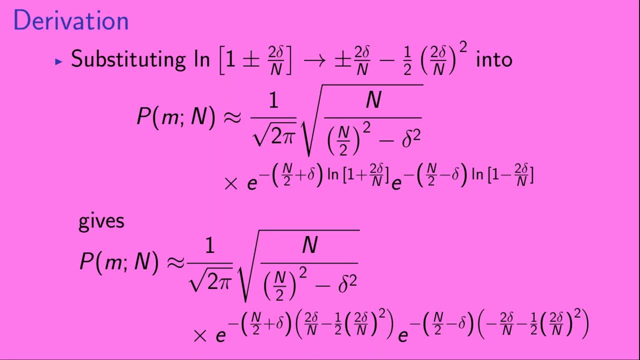 Let's look at the first one. The first one is e to the minus n minus 2.. n over 2 plus delta. natural log of 1 plus 2 delta over n. This becomes e to the minus n over 2 plus delta. times 2 delta over n minus 1, half the. 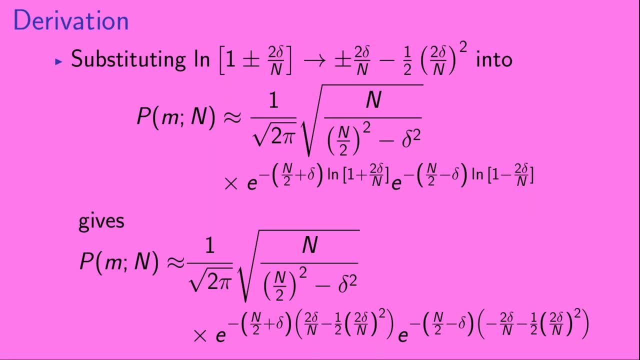 square of 2 delta over n. Now let's look at the second exponential. This is e to the minus n over 2 minus delta. Natural log of 1 plus 2 delta over n. This is e to the minus n minus 2 delta over n. 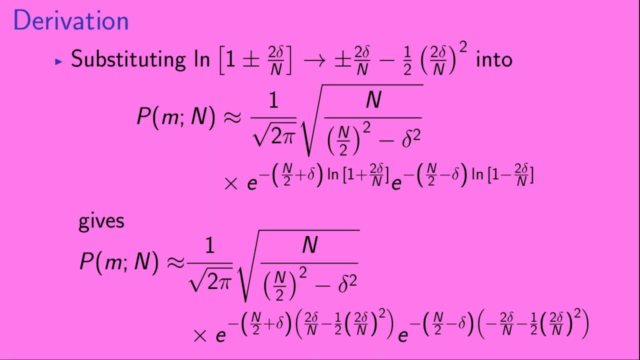 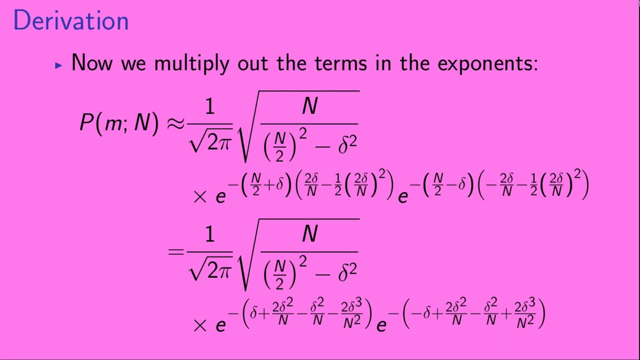 This becomes e to the minus n over 2, minus delta times. minus 2 delta over n. minus 1, half the square of 2 delta over n. Next we're going to multiply out the terms in the exponents, So let's look at the first exponential. 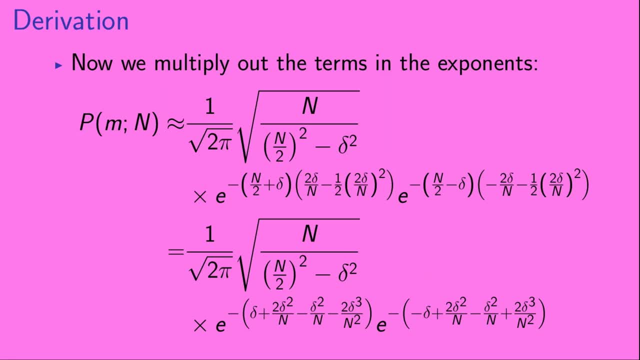 e to the minus n over 2 minus 2 delta over n minus 1 half the square of 2 delta over n n over 2 plus delta times 2 delta over n minus 1 half the square of 2 delta over n. 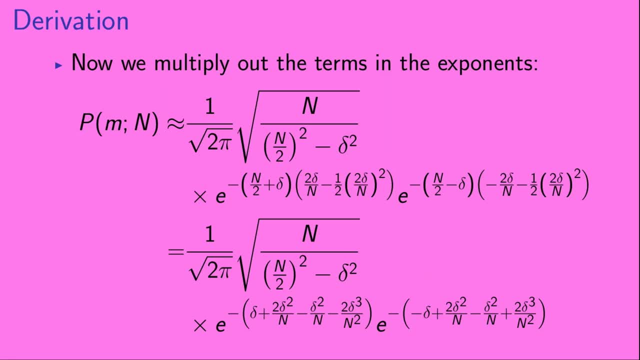 Let's multiply out these terms. So when we multiply n over 2 times 2 delta over n, we get delta. Next, when we multiply the delta times the 2 delta over n, we get 2 delta squared over n. 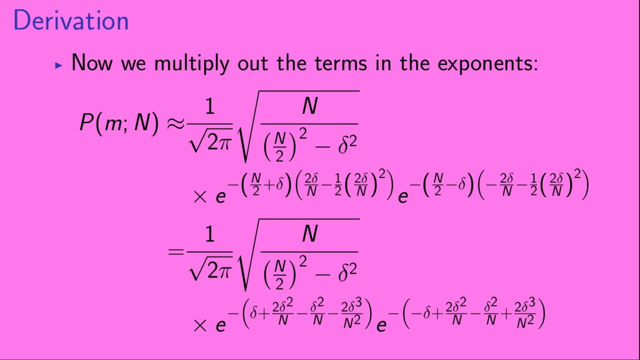 Third, let's multiply the n over 2 times the minus 1, half the square of 2 delta over n. This gives us minus delta squared over n. And lastly, when we multiply the delta times the minus 1, half the square of 2 delta over n. 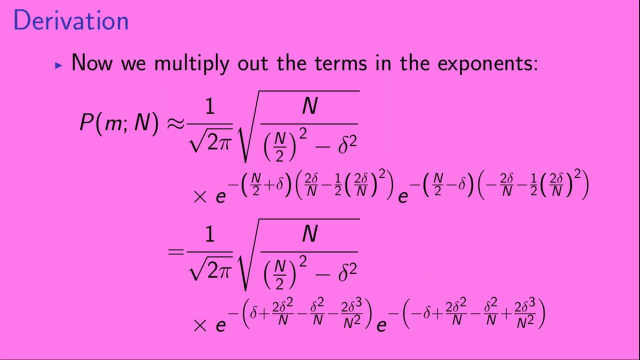 we get minus 2 delta cubed over n squared. So that's it. So that's what happens when we look at the first exponential. When we look at the second exponential, almost exactly the same thing happens, But this time for the first term. instead of getting delta, we get minus delta. 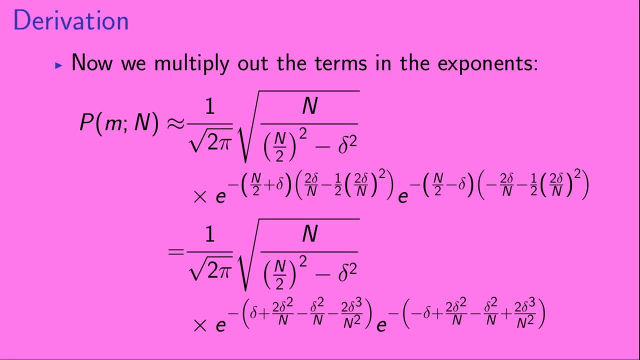 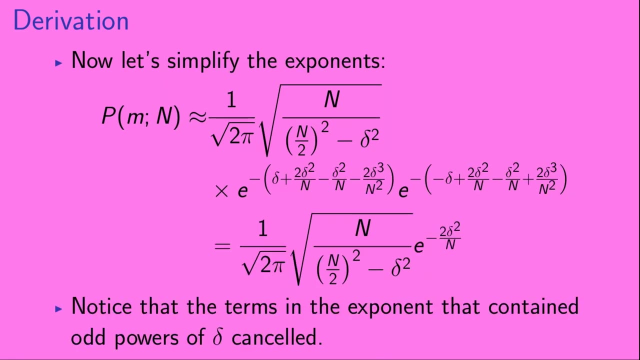 And for the last term, instead of getting minus 2 delta cubed over n squared, we get plus 2 delta cubed over n squared. Okay, now let's simplify the exponents. So again we have these two exponentials. 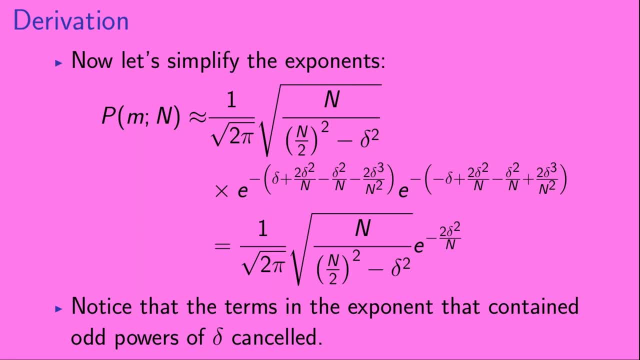 We can see that the first one contains a factor of e to the minus delta And the second one contains a factor of e to the minus minus delta. These will cancel. We can see that the same thing happens with the delta cubed over n squared. 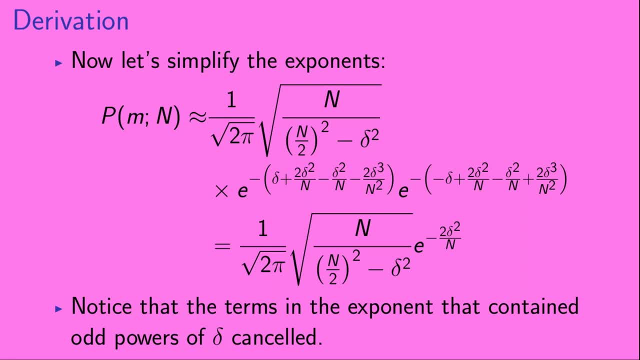 So we have a 2 delta squared over n squared term at the end of each of the two exponentials. So those are going to cancel as well. Now, in the first exponential, we have a 2 delta squared over n, minus a delta squared over n. 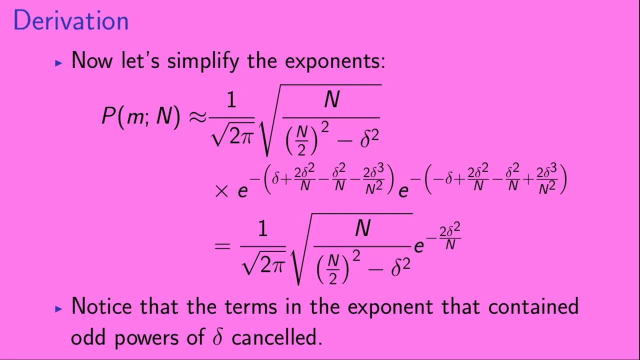 This just gives us a delta squared over n. The same thing happens in the second exponential. So when we multiply these two exponentials together, we just get- We get e to the minus 2 delta squared over n. So notice that the terms in the exponents that contained odd powers of delta have cancelled. 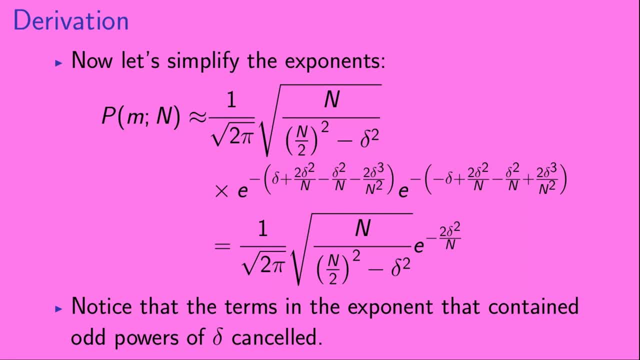 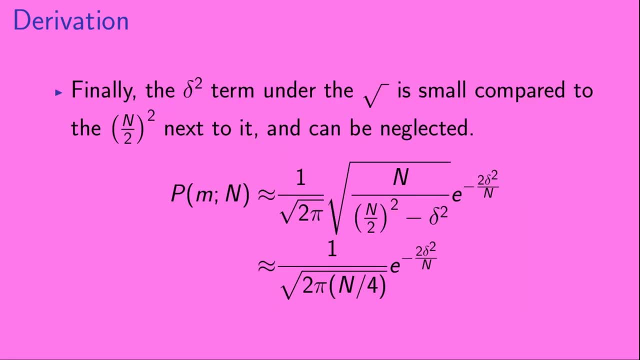 And we can see that, although this calculation has been a long ugly slog, we now have a fairly simple looking result. Finally, the delta squared term under the square root is small. It's small compared to the n over 2 squared sitting next to it and can be neglected. 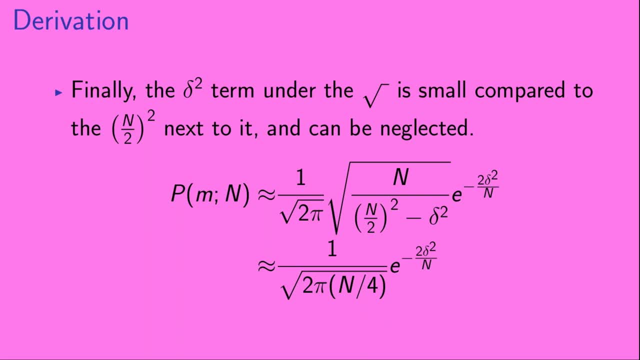 So our expression for p of m given n contained a square root of n over n over 2 squared minus delta squared. This can just be replaced with a square root of 1 over n over 4.. And so we get that p of m given n is approximately equal to. 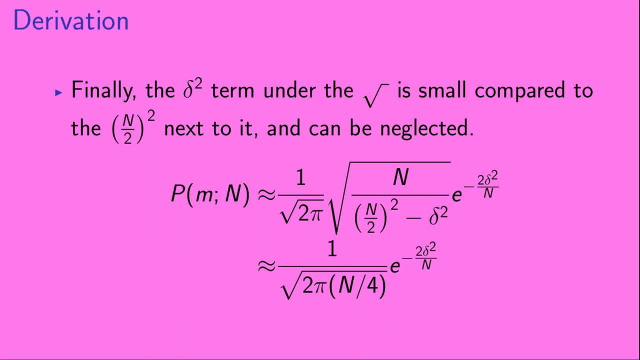 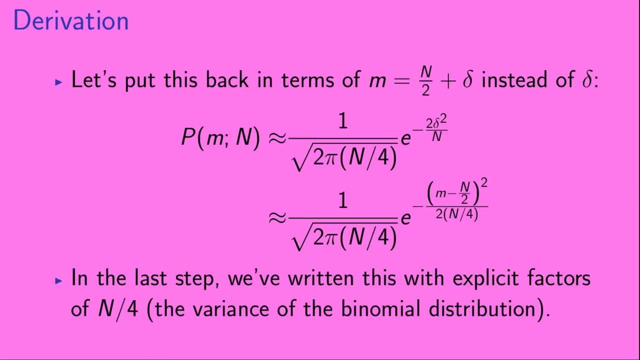 1 over 3.. So we get that p of m given n over the square root of 2, pi, n over 4, e to the minus 2 delta squared over n. Now let's put this back in terms of m, which equaled n over 2, plus delta instead of delta. 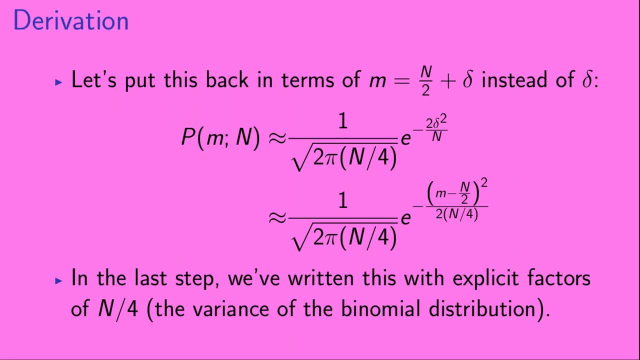 So we just take the exponent in our expression for p of m, given n, which was e, to the minus 2 delta squared over n, and we replace the delta squared over n with the square root of 2 pi n over 4.. 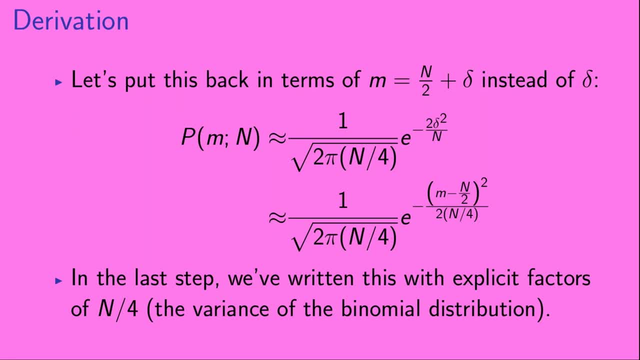 We additional 2 times the alpha squared with m minus n over 2 squared, So we get that p of m given n is approximately equal to 1 over the square root of 2 pi n over 4 e to the minus m minus n over 2 squared over 2 n over 4.. 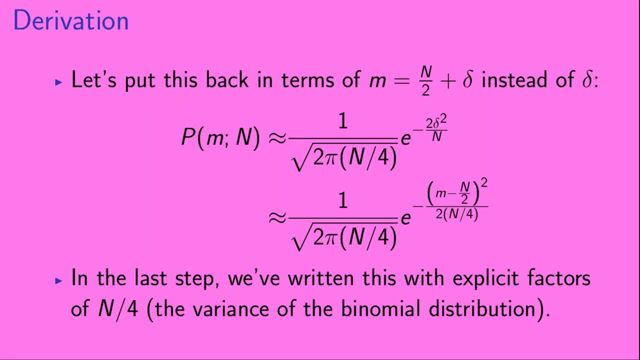 Now, in the last step, we have written this with explicit factors of n over 4.. Which is the variance of the binomial distribution, so that way you can compare this expression to expressions shown in some of our binomial distribution videos, if you like. 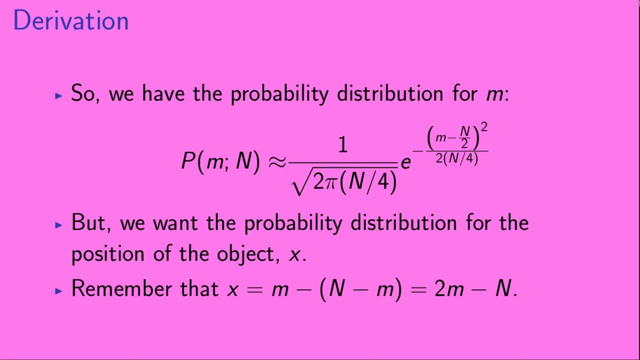 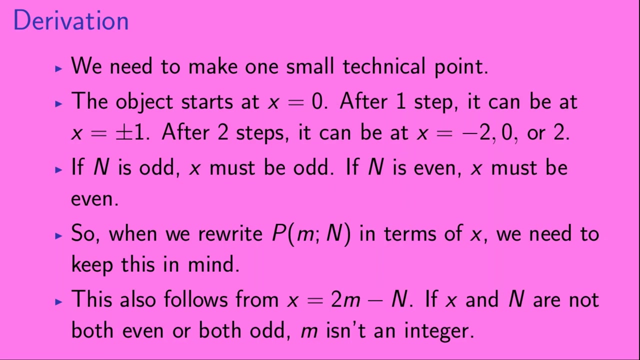 So we now have our probability distribution for m, P given n, but we want the probability distribution for the position of the object x. So remember that x equals m minus n minus m, which equals 2m minus n. Now we need to make one small technical point. 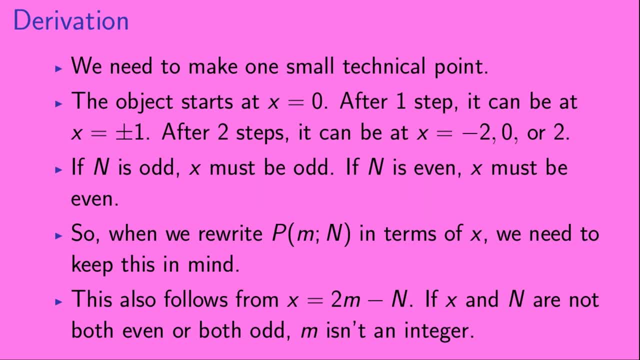 The object starts at x equals 0. After one step, it can be at x equals plus or minus one. After two steps, it can be at x equals minus 2, zero or 2.. If n is odd, x must also be odd, and if n is even, x must also be even. So when we rewrite p of m given n, 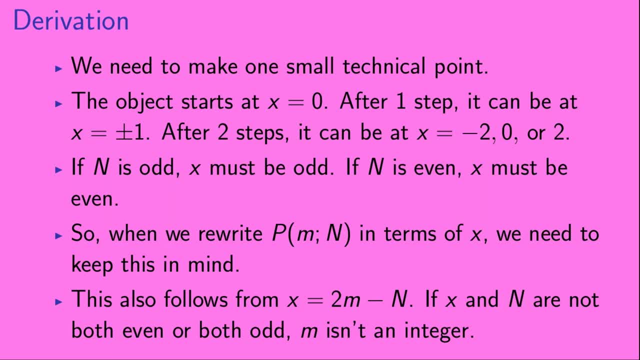 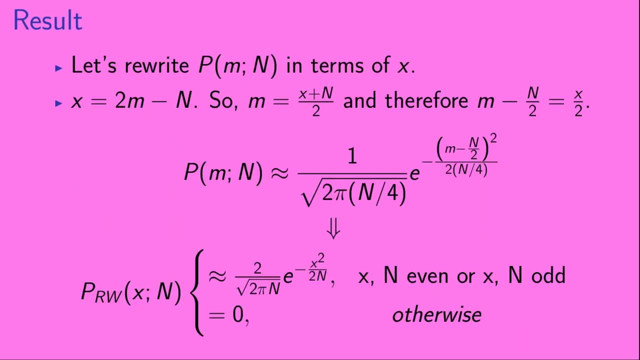 in terms of x. we need to keep this in mind. This also follows from the fact that x equals 2m minus n. If x and n are not both even or both odd, m isn't an integer. Okay, so let's rewrite p of m. 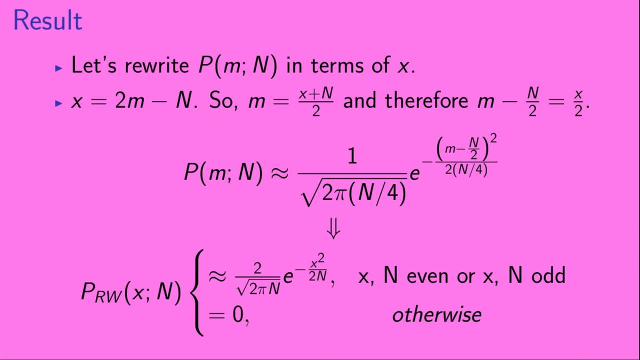 given n in terms of x, So x equals 2m minus n. This implies that m equals x plus n over 2, and therefore m minus n over 2, equals x over 2.. Okay, so, given that we can rewrite our expression for p of m given n, 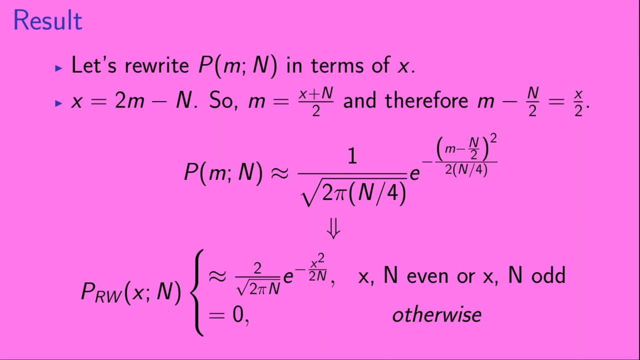 First let's look at that factor out front, the 1 over the square root of 2 pi n over 4.. We can write this more simply by taking that 4 out of the square root and replacing it with a 2 up top, So that factor becomes 2 over the square root of 2 pi n. 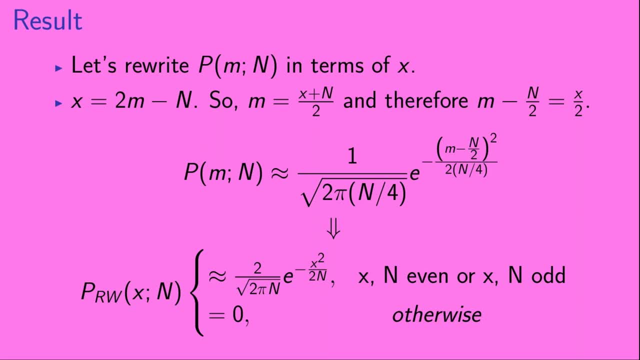 Next we can write the expression for p of m given n. So let's look at that factor out front. we can look at our e to the minus m, minus m over 2, squared over 2n over 4.. Now m minus n over 2,. 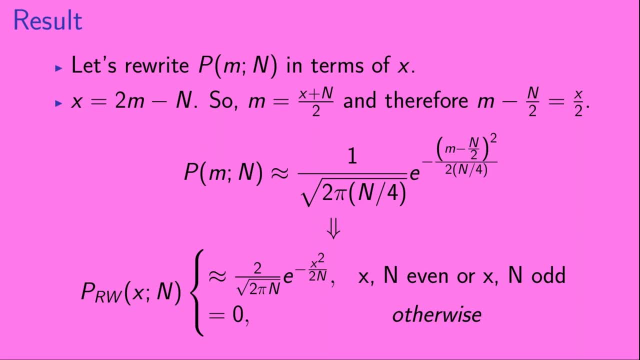 we just said is equal to x over 2.. So this becomes e to the minus x over 2 squared over 2n over 4.. And that simplifies down to just be e to the minus x squared over 2n. So now we can rewrite: 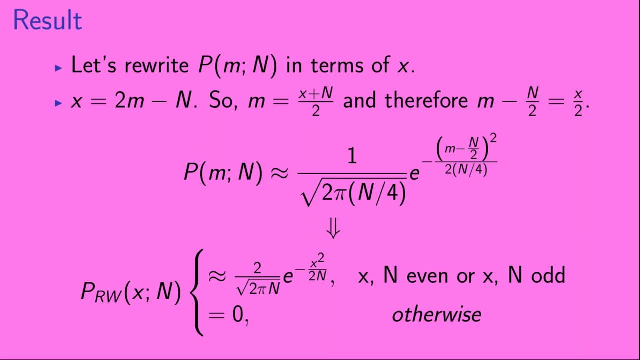 expression in terms of x, and we're going to call this P R w of x given n. So if x and n are both even, or x and n are both odd, P R w of x given n is approximately equal to 2 over the square root of 2 pi n e to the minus x squared over 2 n. And. 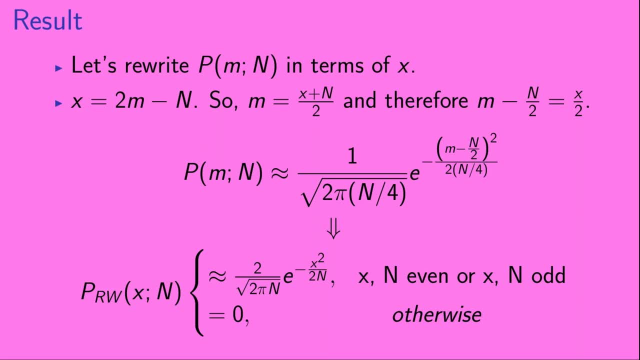 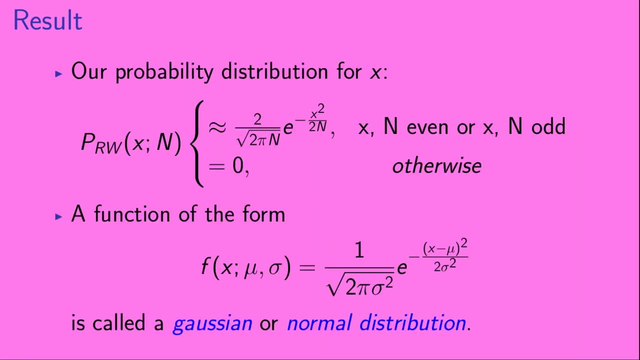 if x and n are not both even or both odd, then P R w of x given n is equal to 0.. So now we have our probability distribution for x, P R w of x given n. Now a function here written as f of x, given mu and Sigma of the form 1 over the square root. 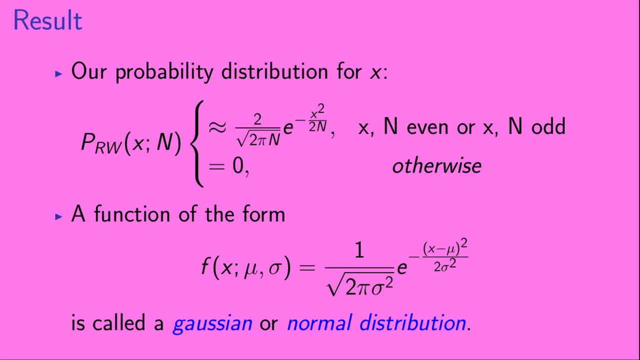 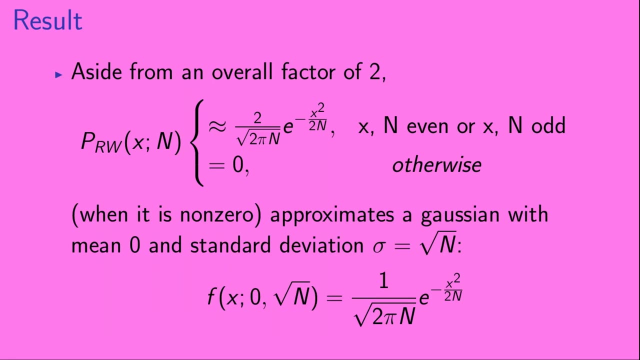 of 2 pi n. So if x and n are both even or both odd, P R w of x, given n is approximately equal to 2 pi sigma squared. e to the minus x, minus mu squared over 2 sigma squared is called a Gaussian or normal distribution. Aside from an overall factor of 2, our probability. 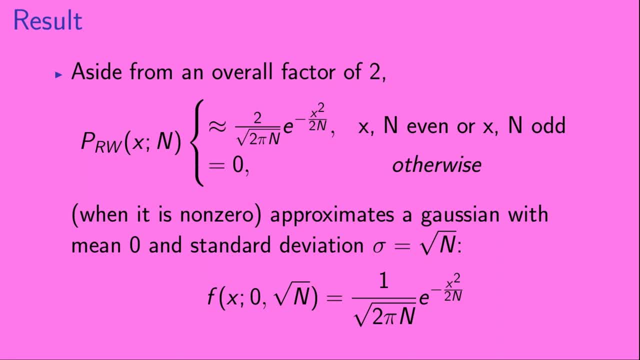 distribution for x, when it is nonzero, approximates a Gaussian with mean 0 and standard deviation sigma equals the square root of n. So here f of x, given n, is equal to 2 pi sigma squared e to the minus x, minus mu squared e to the minus x squared over 2 n, And aside from a factor of 2, that looks just like our. 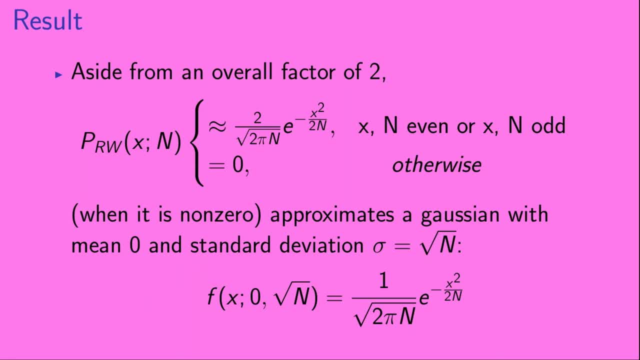 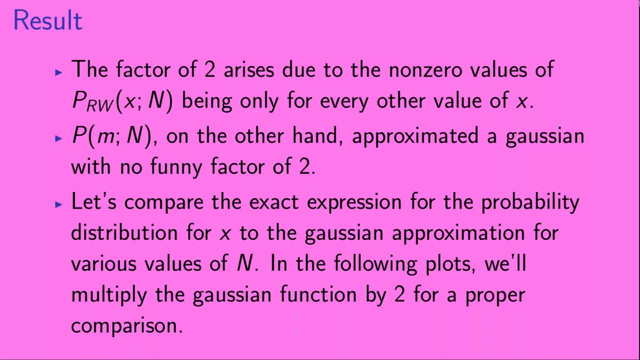 expression for P R w of x given n when it isn't zero. The factor of 2 arises due to the fact that the nonzero value of x given n is equal to 1 over the square root of 2 pi n. So if x and n are both even or both odd, P R w of x given n is equal to 1 over.